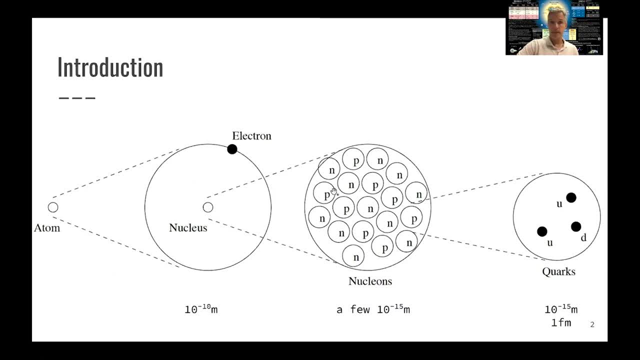 As you see nicely here in this picture, the nuclei can be built out of many neutrons and protons, And even those protons and neutrons are not fundamental particles. A proton, for example, as depicted here, has three components or three constituents, two up quarks and one down quark. A neutron then is built out. 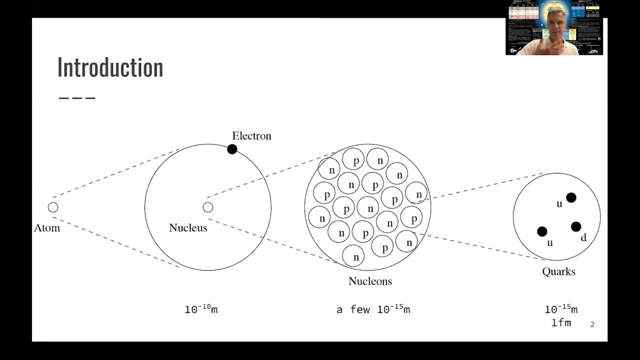 of one down quark and two up quarks. It is kind of important to understand and appreciate the size of those particles, specifically the difference in size, comparing here an atom, a typical atom of the size of 10 to the minus 10 meters, And that compares to a nucleon which can 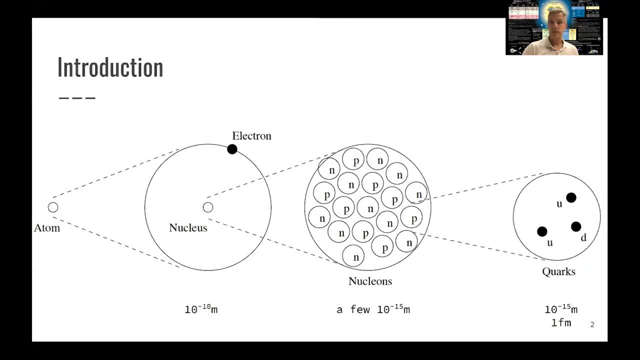 be a few 10 to the minus 15 meters. When we talk about a proton, we typically like to use units of femtometers, which is 10 to the minus 15 meters. So the tremendous size difference also explains the finding of the famous gold foil experiment. 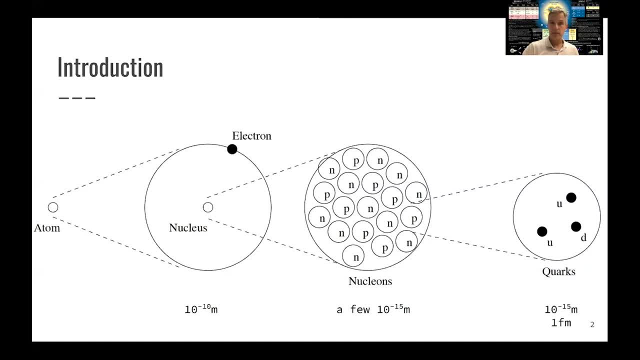 which found that an atom, basically, is made out of nothingness- empty space and a very dense charged core, the nucleus. So you see this very much in this picture and by comparing these order of magnitudes Not shown in this picture, here is a particle which doesn't really like to interact with. anybody else or which the forces is in the manner of the same order. But you can see that there is a tiny, tiny thing which is actually a particle, which is very similar to the particles, Maybe a nice nice particle, But it's something else. It's something else, It's not something else. 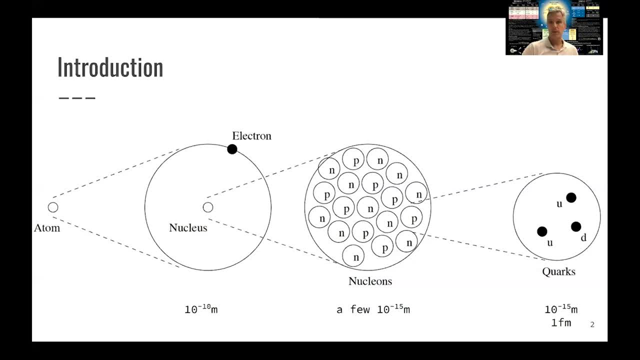 which the forces it's interacting with are so weak that it cannot be bound, And that is the neutrino. A neutrino is not that different from an electron or from a quark, It's just that the interactions it participates in are only the weak force as we understand today. Just to be clear: when I talk about a fundamental particle, I talk about a particle which has no size. It's infinitely small. It has no substructure, meaning it cannot be broken up in constituents, And it can also not be excited. 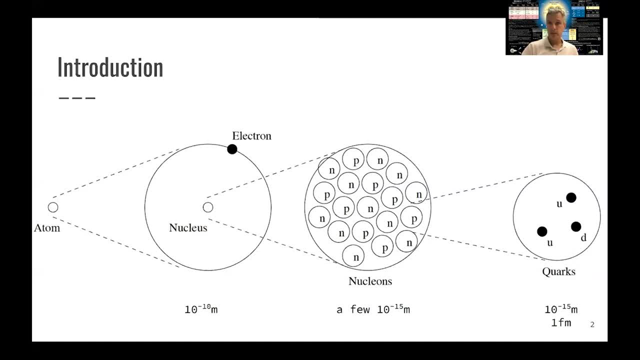 Having said that, this is our current understanding of nature and of those particles. Experimentally, we can only probe those particles to a certain scale or size, And we'll talk later About how precisely we actually do know that a quark is fundamental or an electron is fundamental. 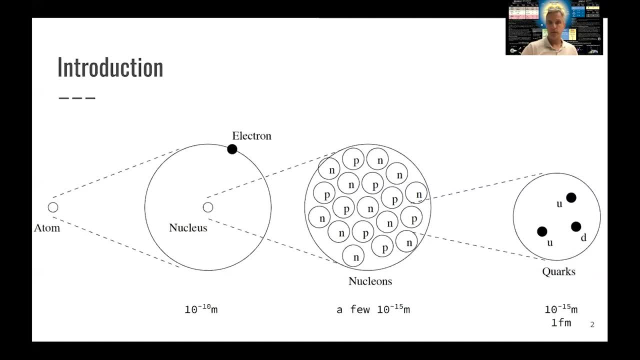 In this discussion here in most of the lecture, I'll talk about the standard model in particle physics. It is a fact that our measurements and our experimental findings are in fantastic agreement with this very predictive theory. The only experimental deviation from this is the fact that we measure the mass of neutrinos to be non-zero. 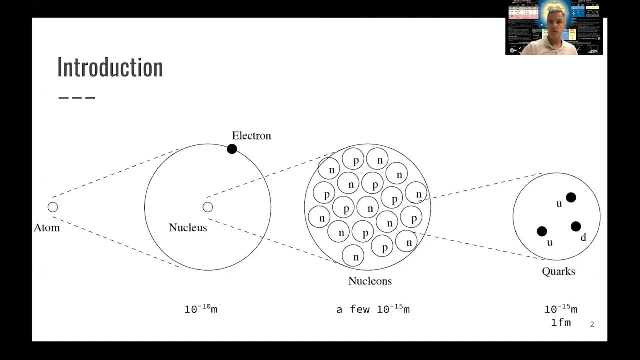 As a consequence, you could say the standard model is broken or we found physics beyond the standard model. But it is actually rather straightforward to extend the standard model to accommodate neutrino masses. So we can just forget about this small fact and assume that the standard model, the standard model, is not Us. 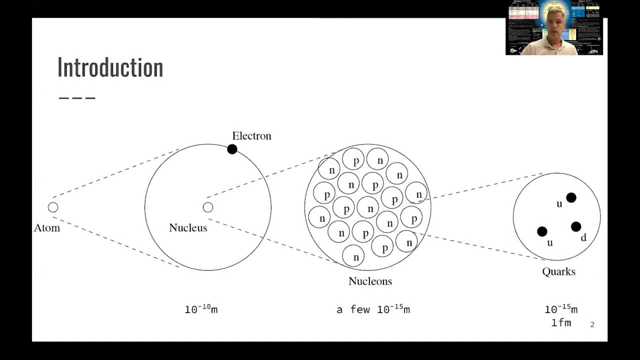 So we can just forget about this small fact and assume that the standard model, the standard model is not Us, assume that the standard model describes nature as we know it. In the last week of this class, we'll talk about motivation, why we think that the standard model. 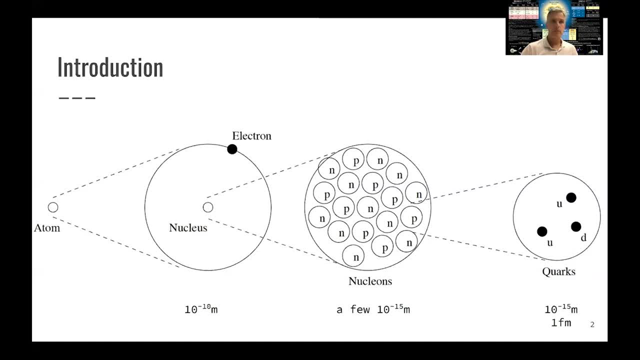 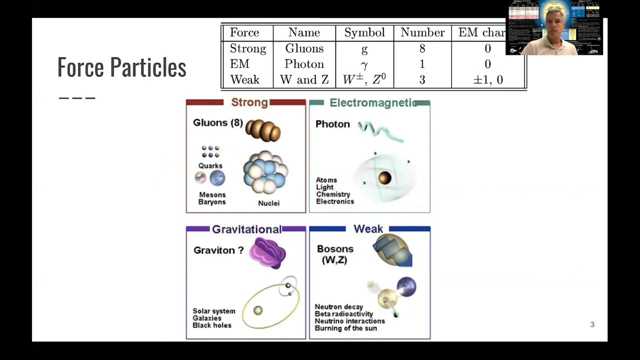 in fact is not complete, And one of the big drivers here is the fact that we cannot describe all of the observations in nature, specifically the observation of dark matter, with the standard model in particle physics. But that's for a later day, Looking into some more detail, the standard model. 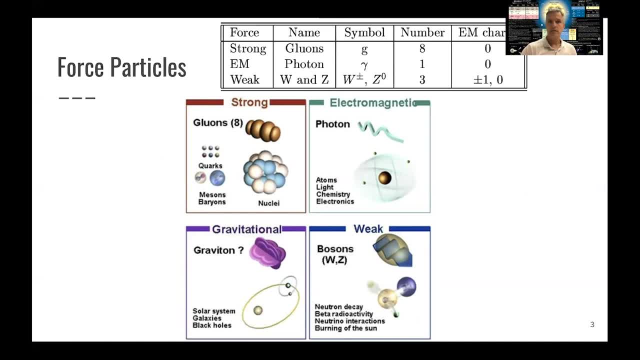 has sets of particles. Some are particles which carry forces and some are metaparticles. The ones who carry forces are all spin-1 particles and there are bosons with that. We have, in the standard model described, three interactions. 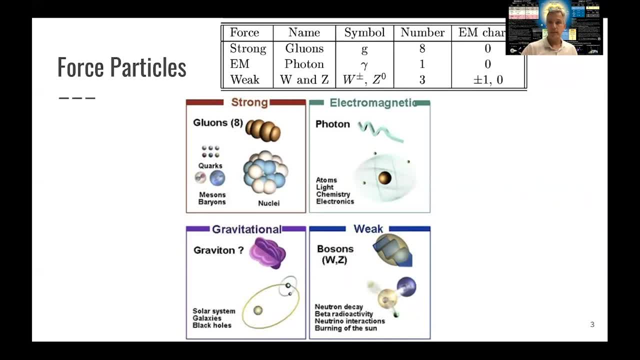 The electromagnetic interactions which you all know from light Electromagnetic phenomena, Chemistry. the atom's behavior or molecule is determined by electromagnetic interactions. Then there's the strong interaction. The name already tells you that it's strong. It's very strong. 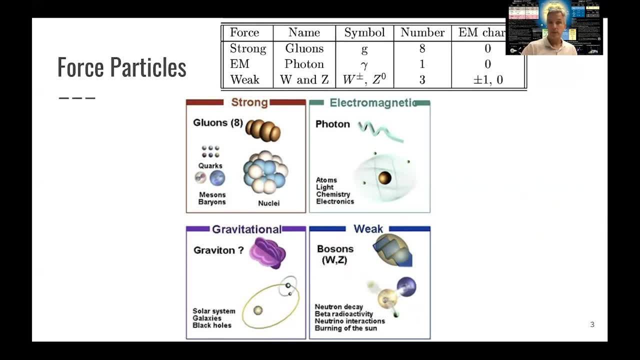 The force carrier here is the gluon. The gluons, there's eight, and they differentiate by the so-called color. It's an interesting effect. And then there is the weak interaction carried by the W boson and the Z boson. 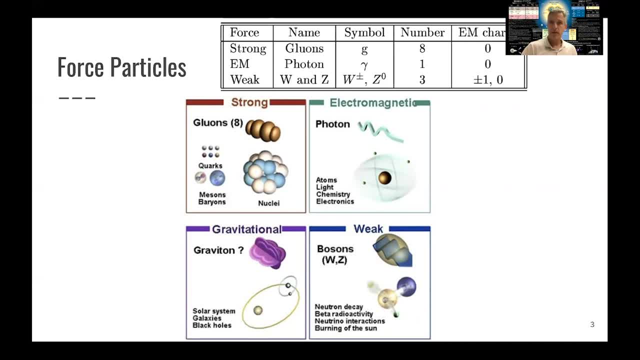 They are different in their own right because they carry mass. They are massive particles and they're actually quite heavy, about 80 to 100 times as heavy as a proton. The weak interaction is responsible for neutron decays, also responsible for the burning of the sun. 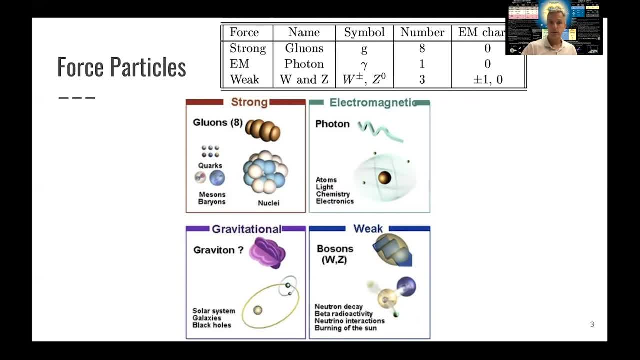 And in our nuclear physics part we'll talk in detail about the weak interaction. We'll talk in detail about what that all means. Gravitational effects are not considered in the standard model. They're very, very weak compared to the strength. 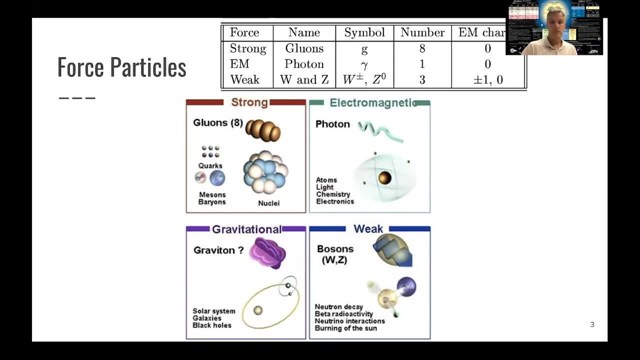 of the other forces we'll discuss here, But it's technically very difficult to actually accommodate gravity as part of a quantum field theory And therefore we will simply ignore this fact, And that's yet another reason why we can consider the standard model to be incomplete. 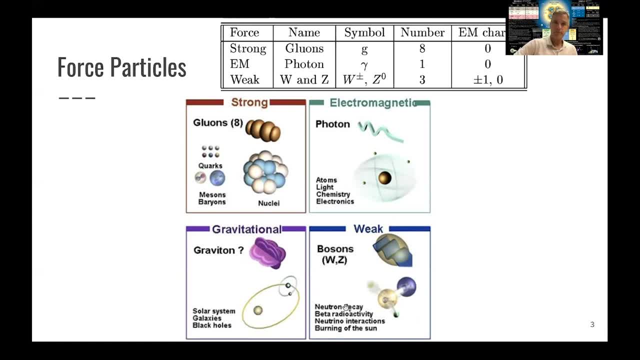 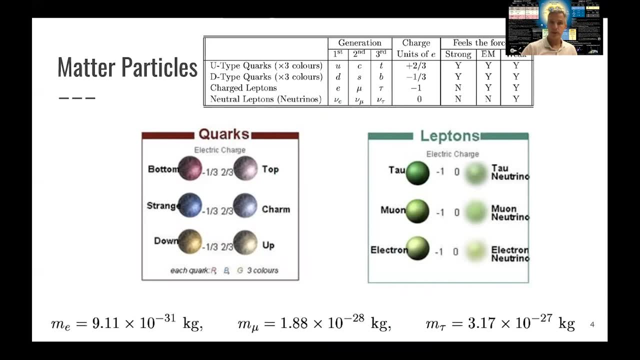 as a model or theory describing nature. The metaparticles themselves are all fermions. They have spin half And they come in three different generations. The only difference between one generation to the next is the fact that those particles have different mass, In other words, their coupling to the Higgs field is different. 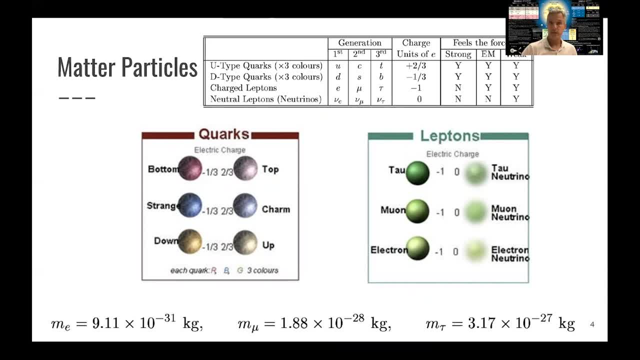 And that's the only difference between those particles. There's consequences out of this. For example, heavier particles can decay. They decay into lighter particles. We differentiate between the quarks and leptons. Quarks partake in the strong interactions, while leptons are neutral in the strong interaction. 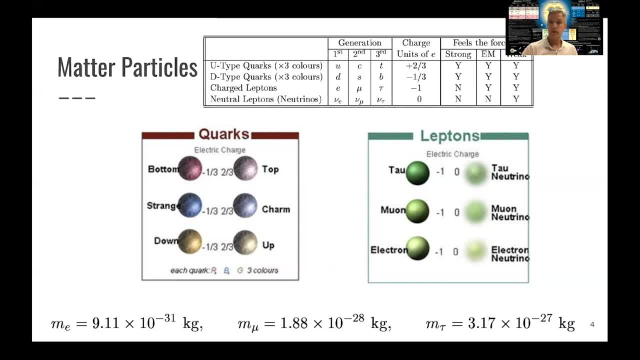 And then we have seen neutrinos already and electron-type particles. Electron-type particles charge leptons. They have electric charge, So they couple to photons, while neutrinos don't. I show you here again one of those striking differences: An electron is 9 times 10 to the minus 31 kilogram heavy. 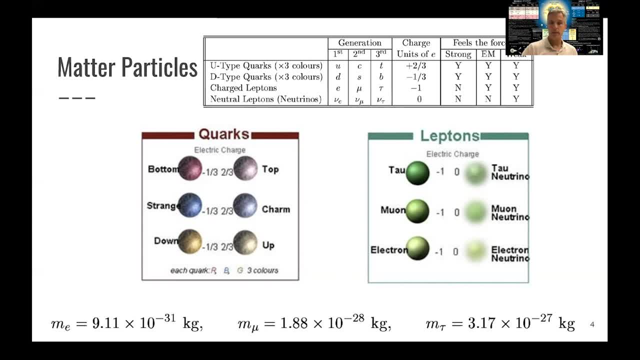 We like to talk about units in a different class, but that's 511 keV, while the muon is about 200 times heavier, and even heavier than the tau lepton And, as I said before, that allows the tau lepton and also the muons to decay into lighter particles. 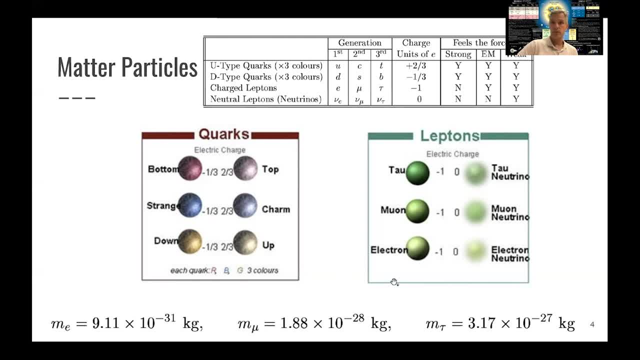 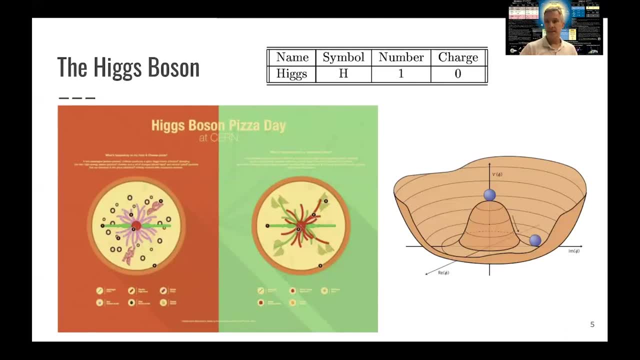 We'll talk about this and how we can use those decays in order to learn about this. And then there's the Higgs boson, And again, the Higgs boson, discovered in 2012, plays a very special role in the standard model. 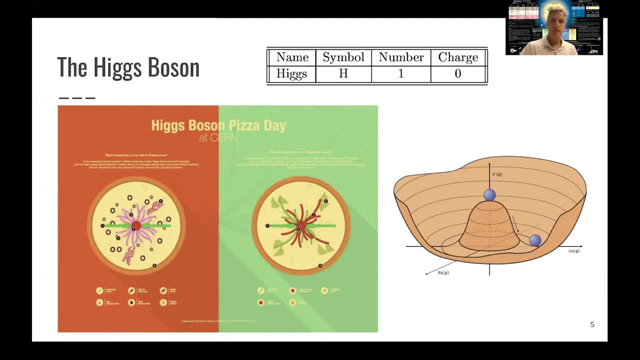 We talk about the Lagrangian, the theory which describes the standard model or which is the basis. There's a theory itself. later on, In this theory we introduce a potential which is shown here at this Mexican head, if you want potential. 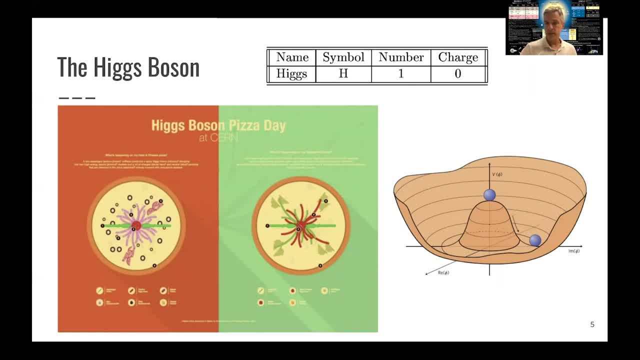 And what you see here is that in this picture, that the lowest energy state of this potential breaks symmetry, So it's away from the zero point, And that symmetry breaking then gives mass to the W and the Z boson which I was describing before. 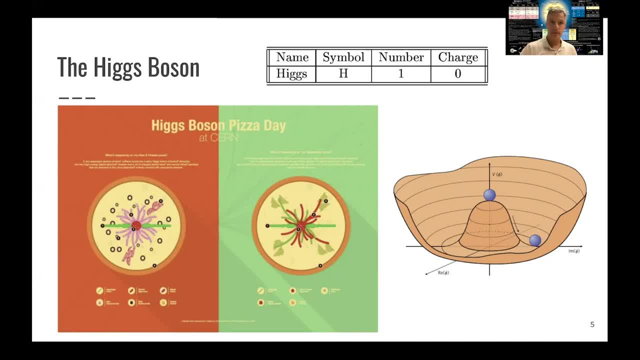 And the coupling of metaparticles to the Higgs field gives mass to those particles. All this on a later date, I thought. here I also give you how CERN actually depicts the Higgs boson. CERN, CERN. July 4th is a special day in the US. 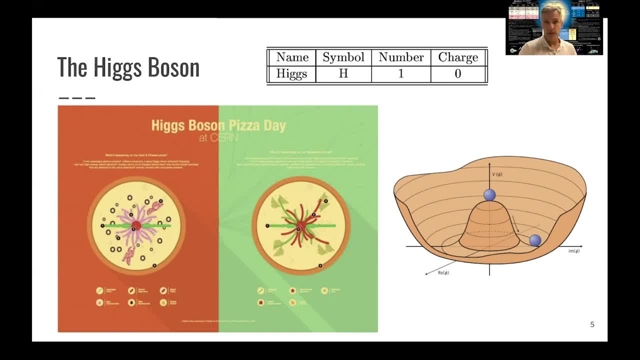 but it's also a special day at CERN, because the Higgs discovery has been announced on this day, And at CERN, typically, the menu is enriched on that day by the Higgs boson itself, in form of pizza which takes the shape of event displays. displays- 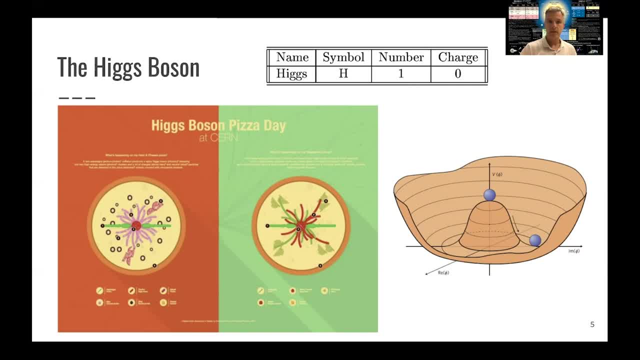 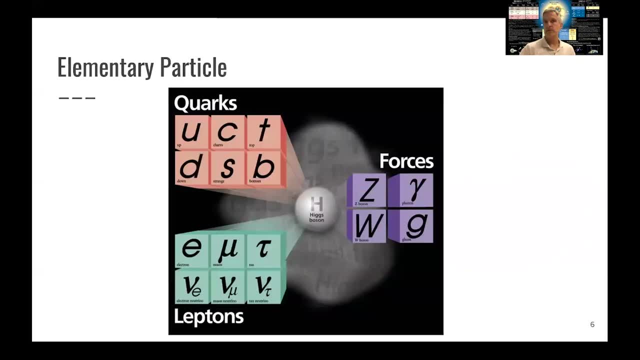 of proton-proton collisions into the Higgs boson and then further decays. We look at some of those event displays also later. So that completes the elementary, the fundamental particles of the standard model, particles which describe almost everything around us. So we have seen the charge in neutral leptons. 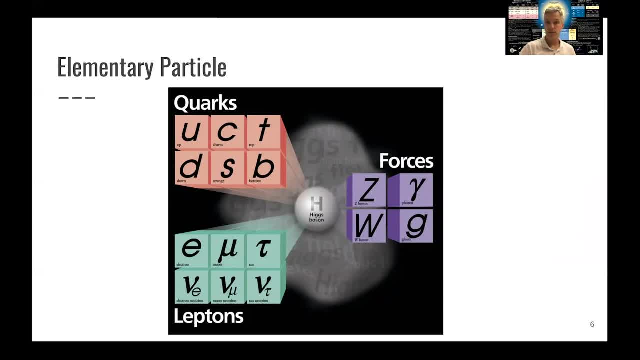 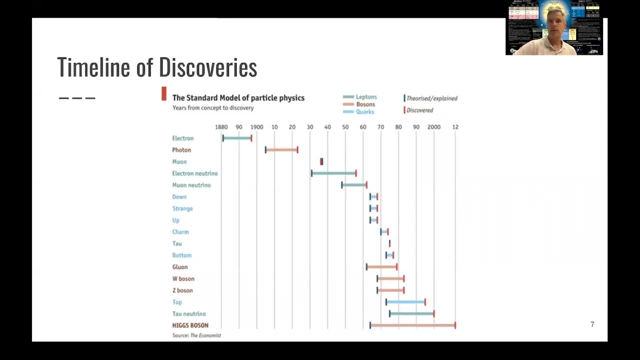 We have seen the quarks, We have seen the force carriers, the W, the Z boson, the photon and the gluon and the Higgs boson, which is kind of the very special particle holding this all together. An interesting point. here is again looking a little bit. 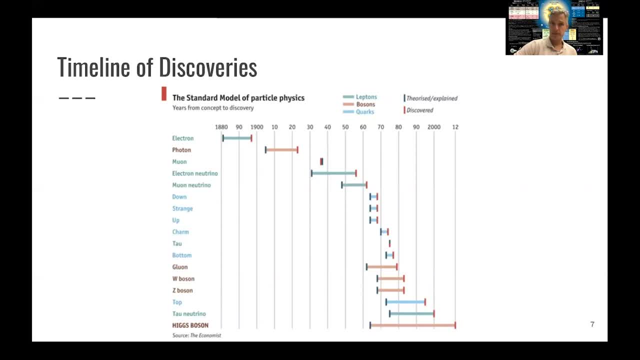 at history and when those particles have been discovered, and also when those particles have been explained- And I don't want to read this all to you- You'd see that the earliest discovery was the discovery by JJ Thomson of the electron and the latest the completion of the particles. in the standard model, the Higgs boson, in 2012.. Interesting for the Higgs boson, the time between the theoretical discovery by Peter Higgs and friends was about 50 years before the experimental discovery. But then there is also composite particles. 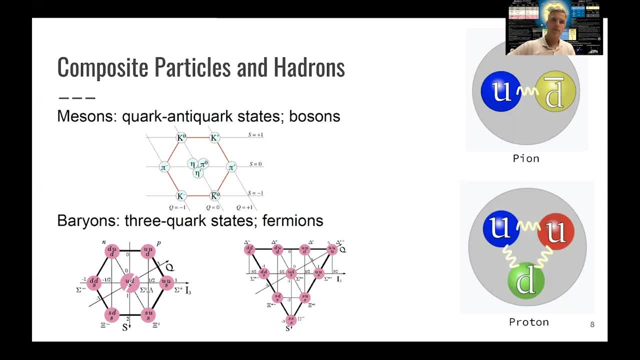 So the things around you are all composite particles. Here we can differentiate between mesons and baryons. Mesons are particles which are made out of quarks and antiquark pairs of a bound state, And they are bosonic because you add in half. 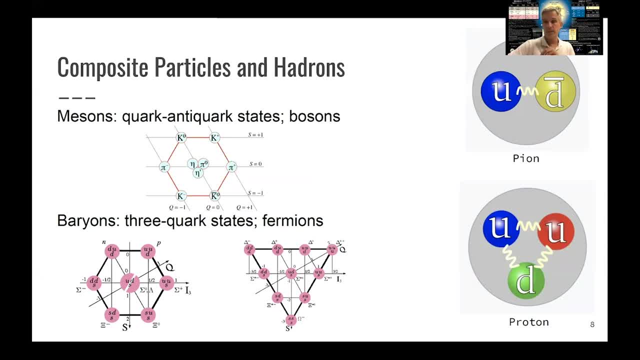 two spin half particles together. One example is a pion which is made out of up quarks and down quarks that can be charged in neutral pions, And the zoo of particle increases quite quickly if you then consider that it's not just up and down quarks. 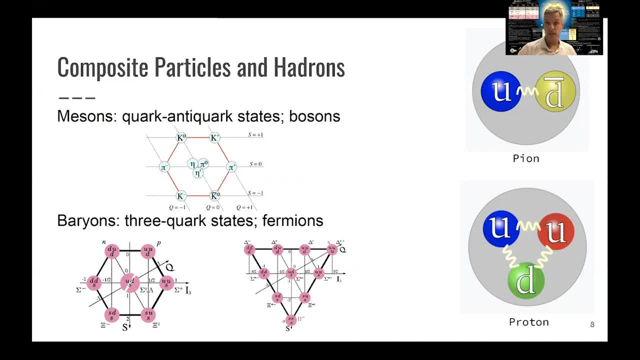 making those particles. but you could add strangeness to that meaning, a strange quark. And so you see here in this picture the mesons, the pions, etters, But also then neutrals and charged particles with different charges, And then kaons, which are particles. 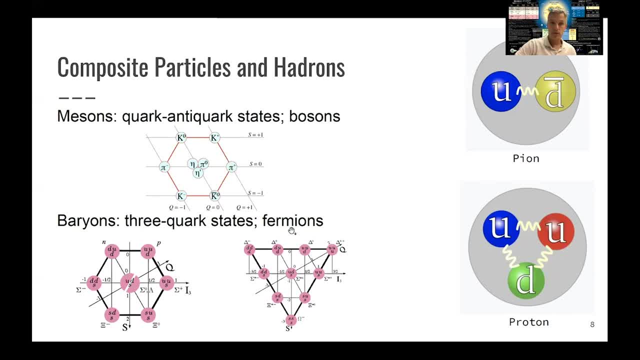 which have one S quark in addition to an up quark and down quark, And then there's baryons. They're made out of three quarks. We have already seen the proton and the neutron, But also here you can see a different configuration. 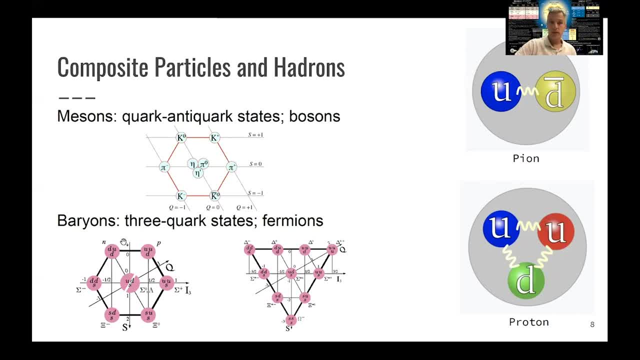 We'll introduce a concept of isospin. You can see here the proton and the neutron, and then strangeness being added with one or two components of strangeness, And then there's this isospin. This is an isospin component as well. 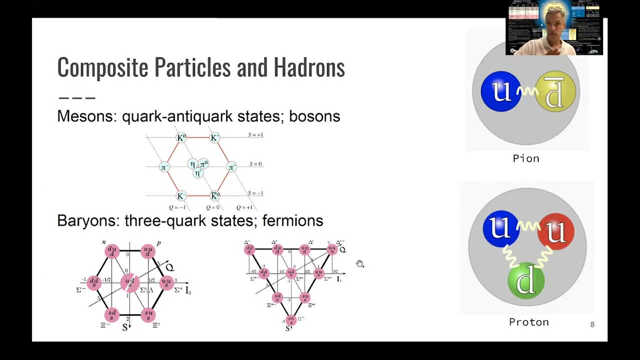 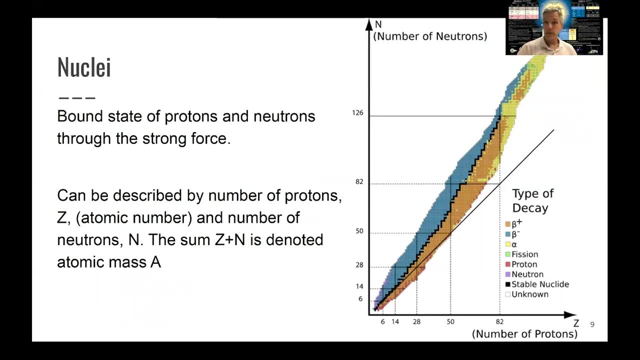 This situation becomes complex very, very quickly, But we'll look at this in more detail. And then again, putting those bound states together- bound states of protons and neutrons through the strong force- gives us a rich table of nuclei on isotope tape. 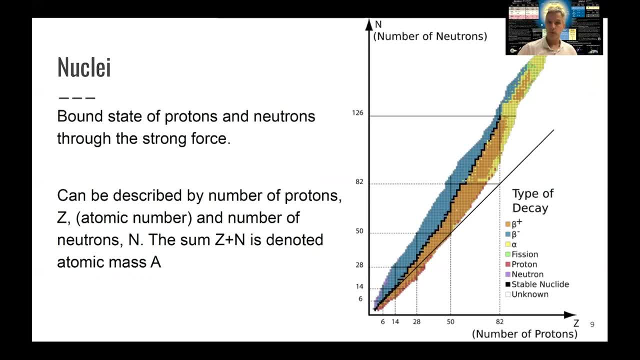 Here you can describe nuclei by the number of protons, which is typically called z, and the number of neutrons, which is typically called n. The sum n by z, This is the atomic mass. Each proton and the neutron are about 1 GeV heavy.